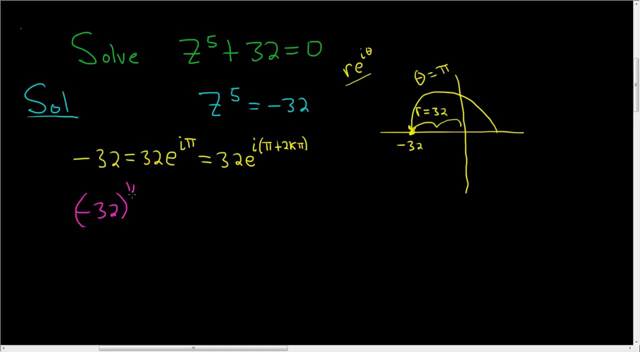 we get negative 32 to the one-fifth, That's 32 to the one-fifth e, and then what we can do is do the following: We can just divide by five. so pi plus 2k, pi divided by five, Super fast way. 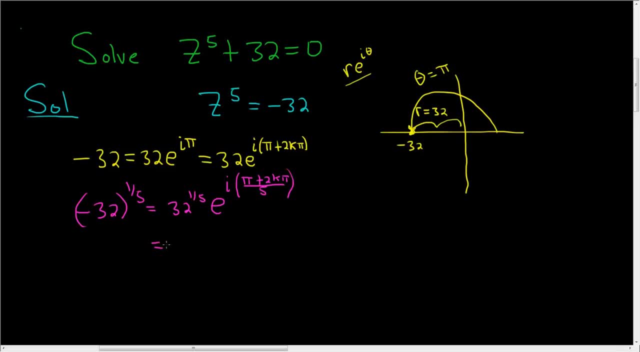 to do. it always works every single time. So this is 2 e to the i pi plus 2k pi over five, And now we can specify values. So we're taking the fifth root, so we're going to have five roots. 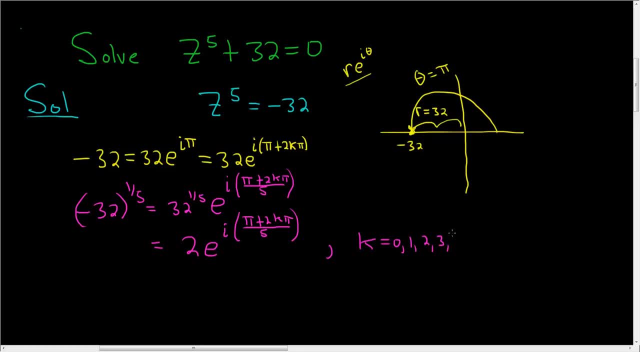 so 0,, 1,, 2,, 3,, 4.. And we just plug in 0,, 1,, 2, and 3, and 4 here and we get all of the roots. So let's go ahead and do it carefully. So when k is equal to 0, we get- let's call it z1,. 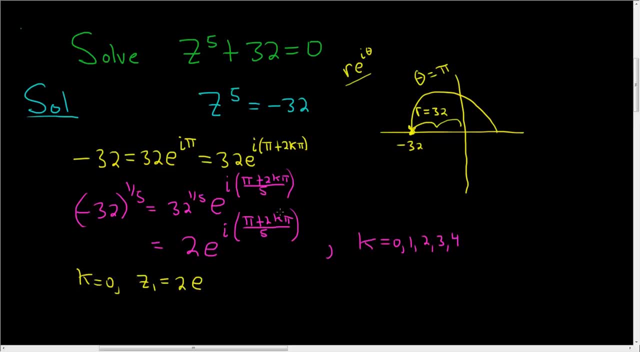 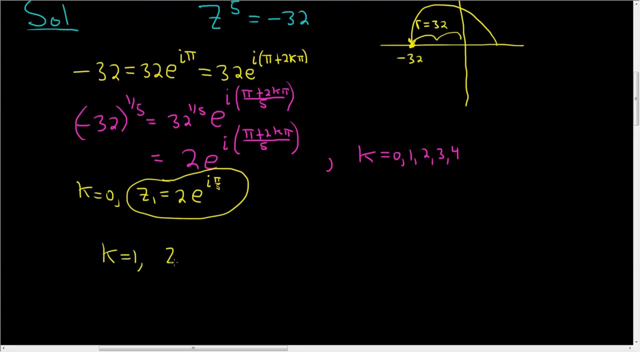 we're going to get 2 e, and then k is 0, so we're just going to get pi over 5.. So e to the i, pi over 5.. So that's one answer. When k is 1, we get z2, and that's 2 e to the i, And let's see: 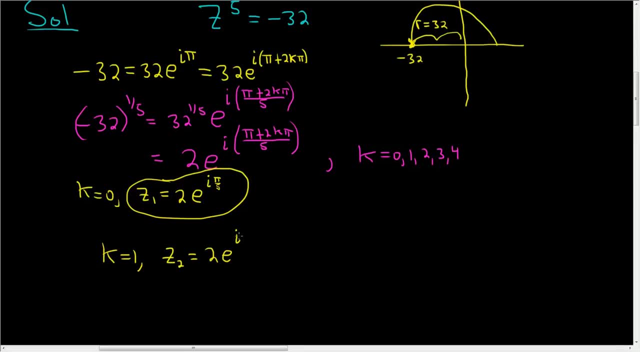 we're plugging in 1, so we're going to get 2 pi. 2 pi plus pi is 3 pi, so we get 3 pi over 5.. So that's another root. When k is equal to 2, we're going to get z3,. 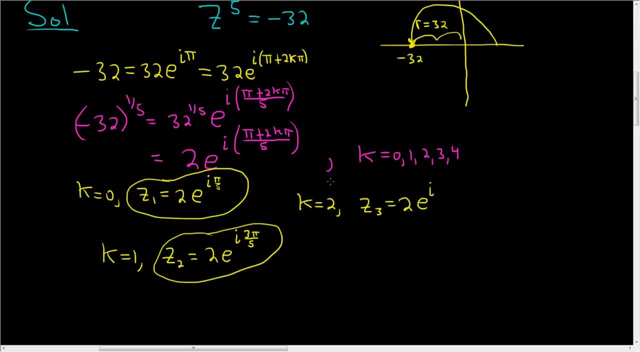 and that's going to be 0.. So that's going to be 2 e to the i. And let's see we're plugging in 2, so 2 times 2 pi is 4 pi. 4 pi plus pi is 5 pi. So we get 5 pi over pi. So that's 2 e to the i pi. 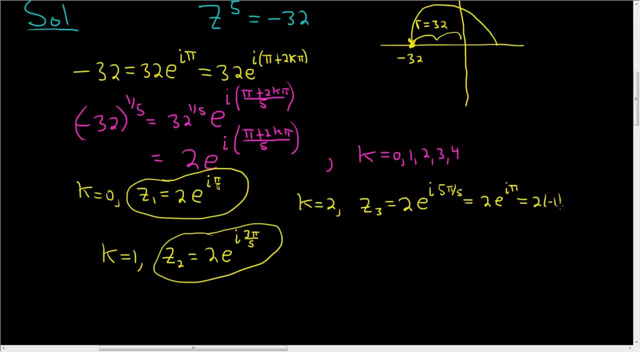 Well, e to the i pi is negative 1, so we get 2 times negative 1,, which is negative 2.. So z3 is negative 2.. And then when k is 3,, again we plug in 3,. 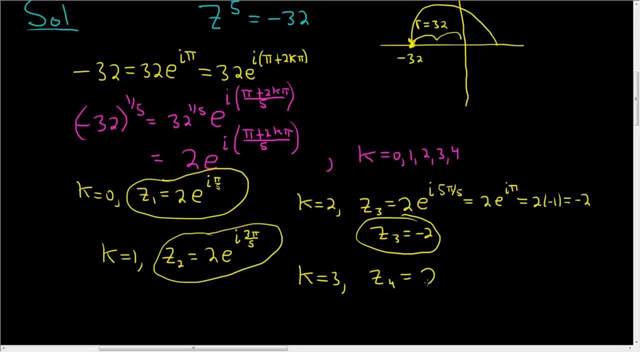 so we get z4 this time. So this is 2 e to the i And we're plugging in 3, so we're going to get 2 times 3 times pi. So we're going to get 6 pi And we're adding that to pi.